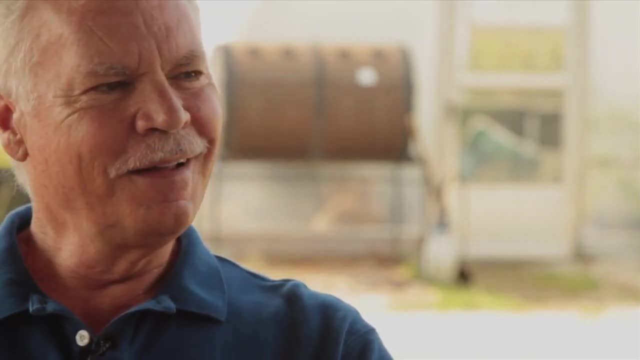 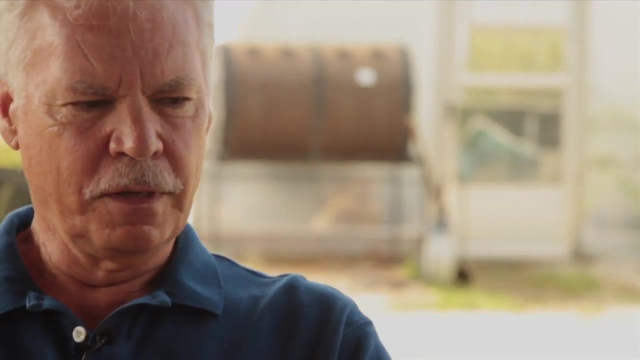 of did a long series of experiments to sort of figure out what was going on, And so the first thing that we wanted to do was to replicate those experiments in the field, And basically what we were doing was we were treating the cucumber seed with these bacteria in a vegetative form. We would make a slurry and you would dip the seeds in the slurry and then you would plant the cucumbers. We did indeed show again that the bacteria that were treated with the cucumber beetles were resistant or tolerant to some degree to the disease. So you know, we knew that. 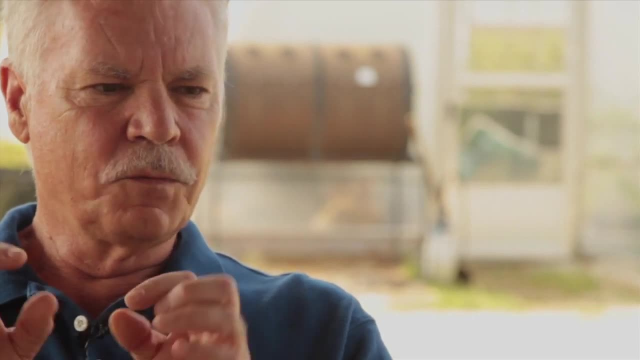 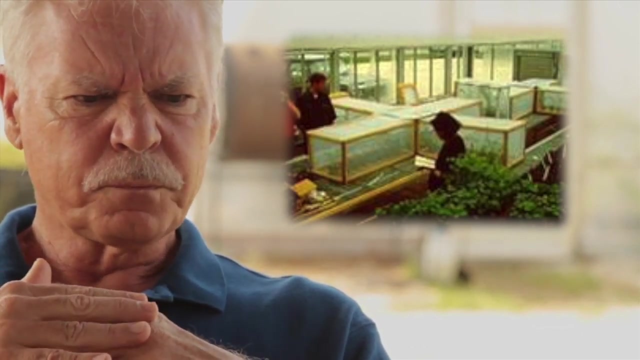 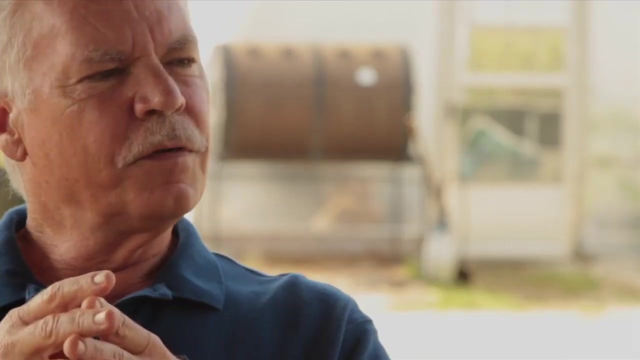 there was something going on. So the next thing that we did was we wanted to focus on the cucumber beetles. So we did some cage experiments in the greenhouse where we built some cages where we could confine the cucumber beetles, And it was very dramatic, the difference in feed. 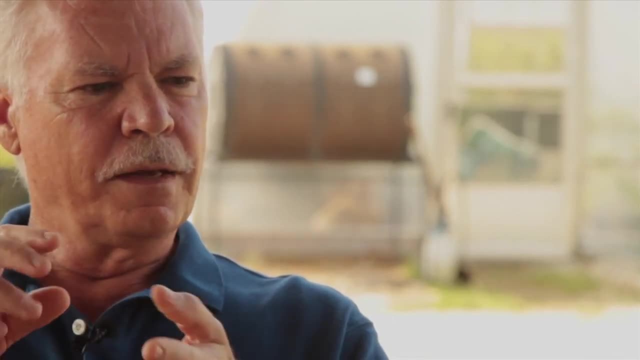 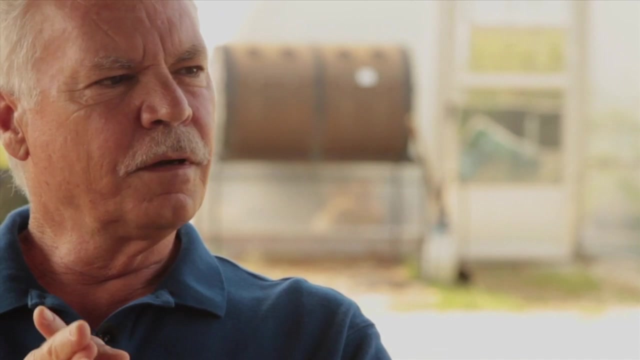 In feeding by the cucumber beetles on the plants. the control plants were just chewed down basically to nothing, And the plants that were treated, you know, had very little feeding damage on them And we also showed that the incidence of bacterial wilt was much. 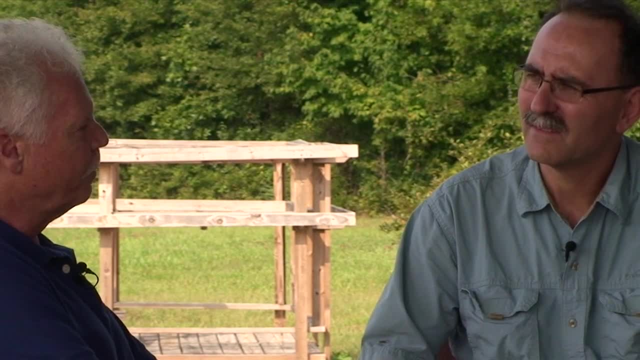 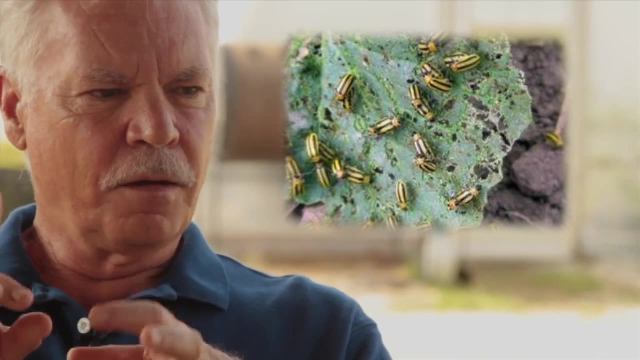 greater in the control plants than on the plants that were treated with the bacteria. Cucumber beetles are fairly unique in that they're stimulated by these plant compounds called cucurbitacin. And so we thought: huh, you know something going on here. And we found that the cucurbitacin 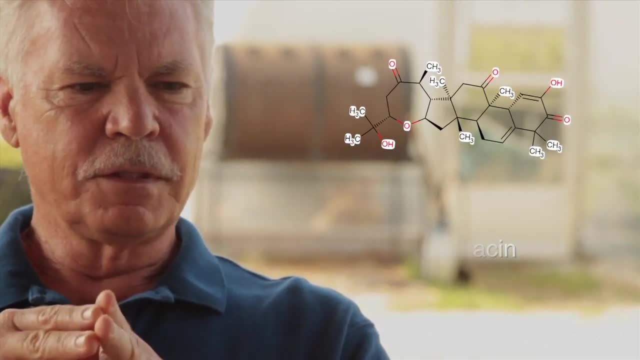 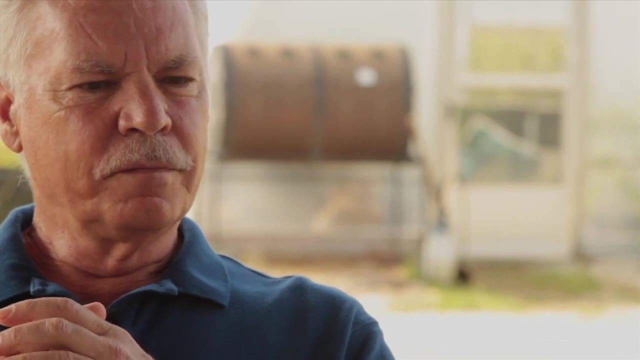 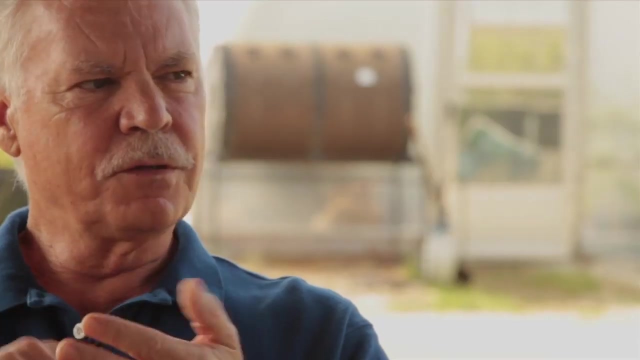 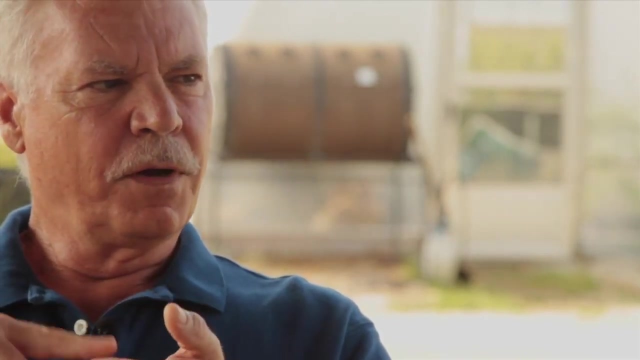 levels were significantly reduced on the plants that had been treated with the bacteria. So that was a significant finding, and we did some literature reviews and found that some of the precursor compounds in the plants for making cucurbitacin are also precursor compounds involved in these plant diseases. 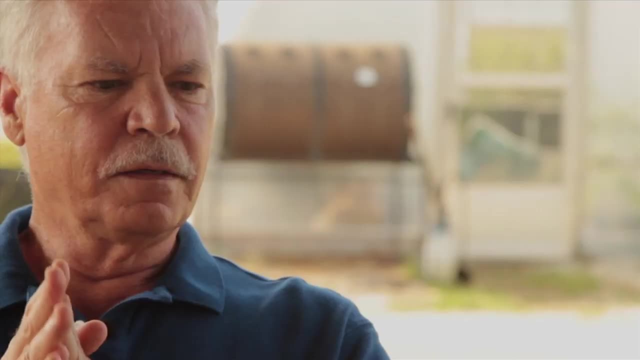 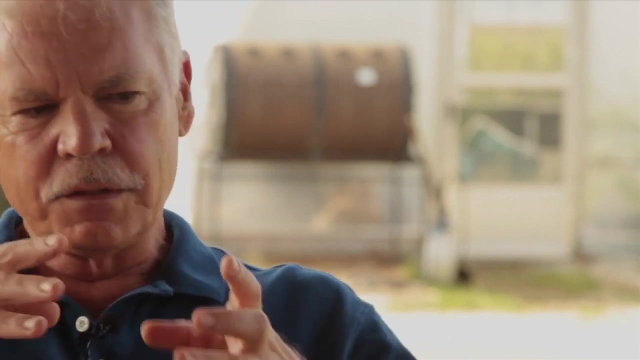 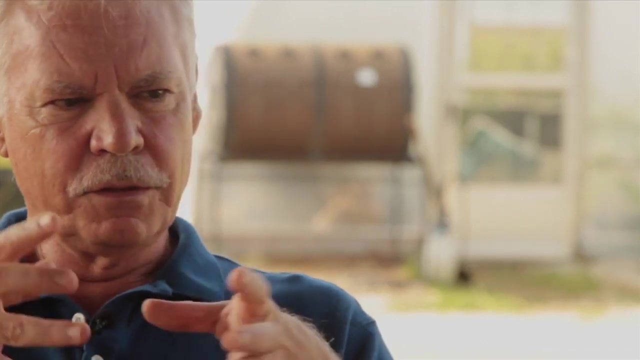 defense pathways. So what we suspect is happening is that if you, you know, treat the plants with the rhizobacteria it's producing, you know it's turning on the plant defense pathways, which is the whole chemical cascade of events in the plant And the plants using those precursor. 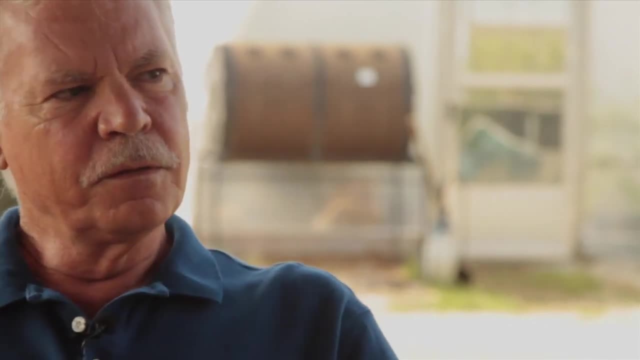 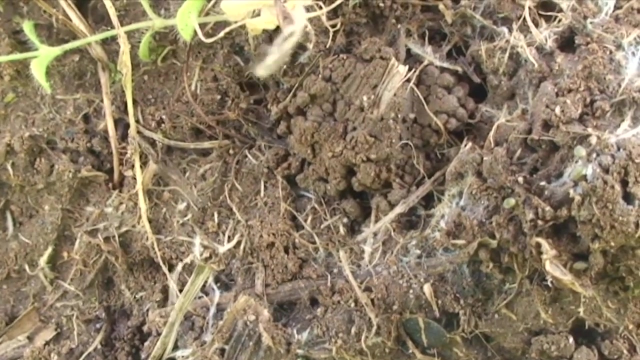 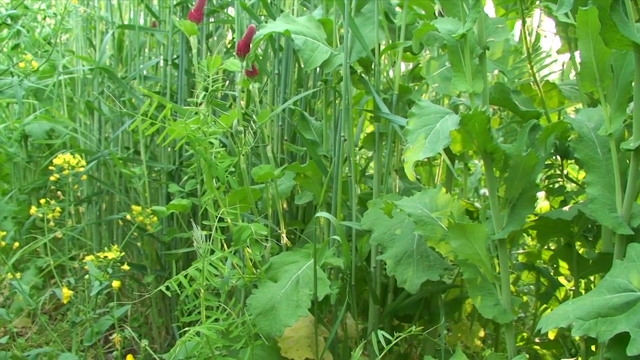 compounds that normally would go into cucurbitacin, into this plant defense pathway. So that's what we think is happening. Okay, The key thing is, you know these bacteria occur naturally, Right? So if farmers can kind of maintain the you know- microbial diversity in the soil,